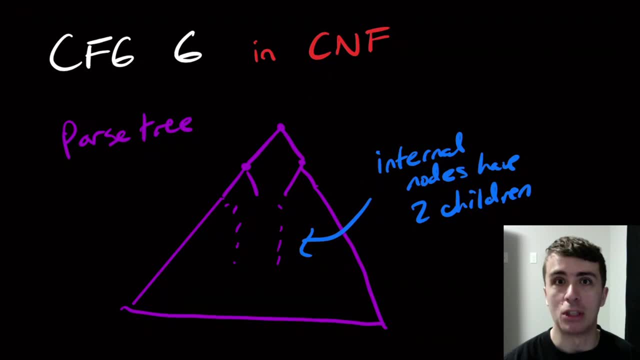 it means that it has two children here, and if we didn't have the grammar of C and F, the right-hand side could be technically anything, so the children underneath a node could theoretically be anything. but restricting it in this form allows us to restrict what the what the parse tree actually looks like. 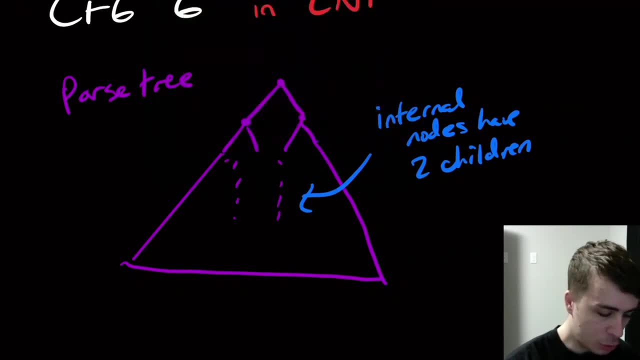 but other than that, at the bottom of the tree we'll have something like: each of these bottom nodes will produce one terminal, because when we read the tree from left to right, at the leaves, we will read all of the terminals of the string that was created, and the reason we chose C and F here was that the other 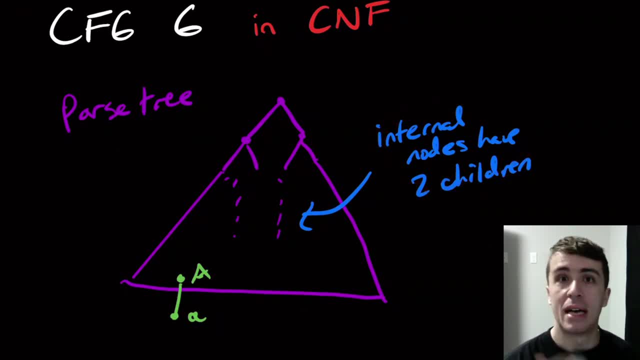 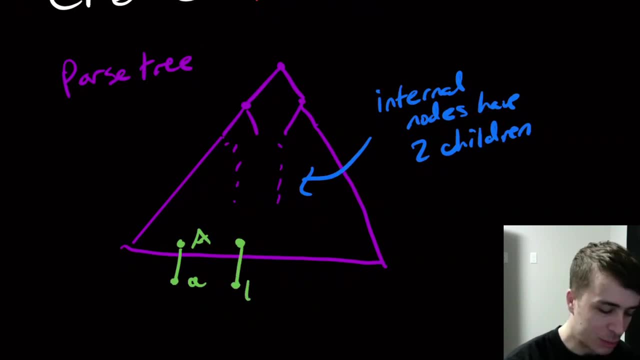 type of rule other than this one was that a variable can produce exactly one terminal, so no one can have one child. so at the very bottom of the tree it kind of looks like Christmas ornaments and some sense that we have a bunch of variables having exactly one child. so all of these nodes right here. so these 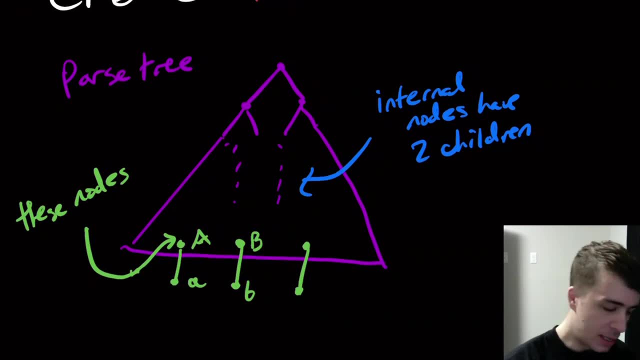 notes. although they're technically internal, I'm not going to consider them internal nodes. these notes have one child and all of the actually leaves the very, very, very bottom of the tree. these have exactly zero children. They're childless because they're terminals And because it's a context-free grammar. we can't replace a terminal. 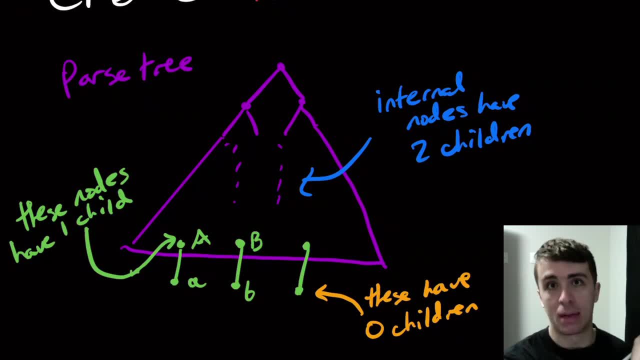 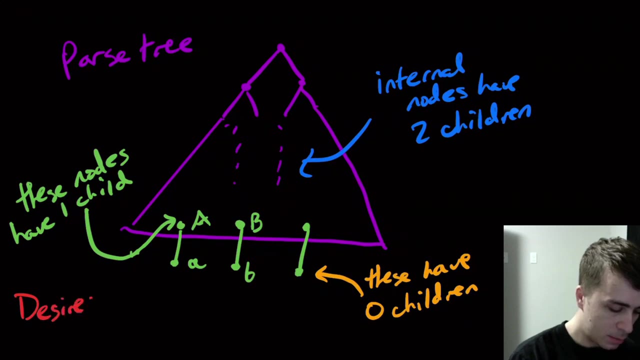 with anything, It's only a single variable with something. In this case, it's either two variables or one terminal. So what we're going to do here is that the desired behavior. so we desire to have the tree so big that we repeat variables going from the top to the bottom. 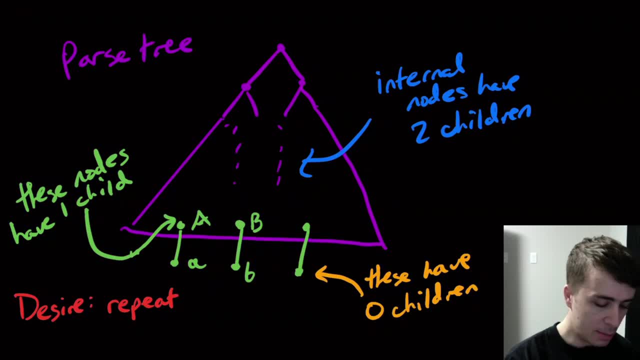 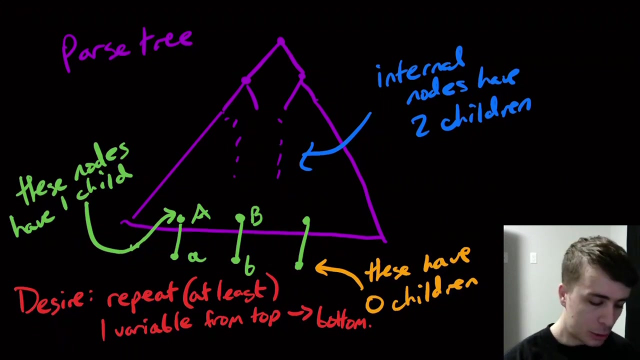 So we want to repeat at least- oops, not least, I'm not renting anything here- Repeat at least one variable From the top to the bottom of the tree, And that gives some kind of repeating behavior, kind of like when we repeated the state in the DFA. So in order for this to actually work, 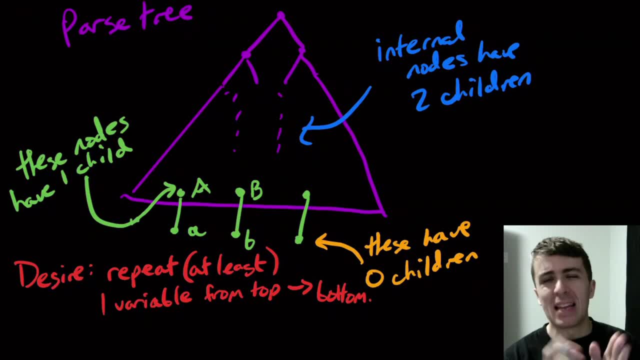 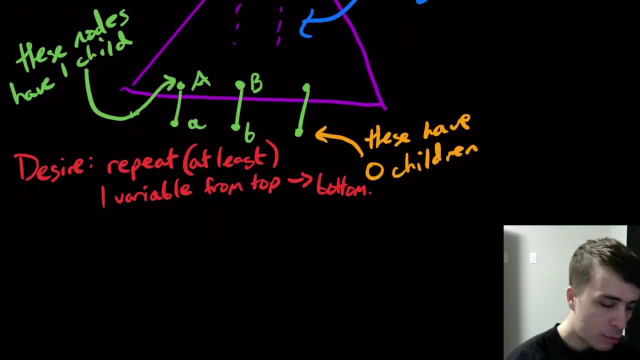 if the tree is kind of short, meaning that the string that we're trying to create is short, meaning that the tree is short, then it could theoretically be that there's no repetition of a variable going from the top to the bottom. So all that we really need is that we need to consider one specific path. 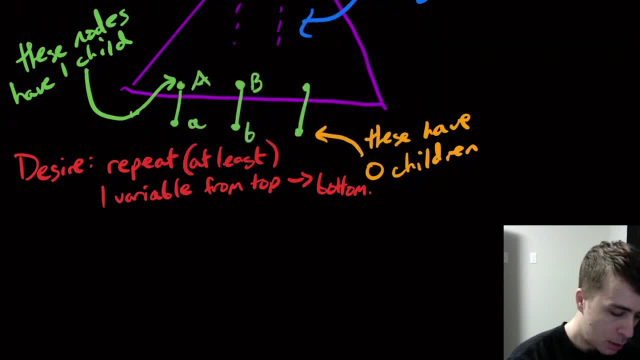 going from the top to the bottom. So to do this, we need to ensure that the longest- so as long as the longest one has some kind of repeat in here, it's OK, It doesn't actually matter, But we need to have at least one of the ways from the top to the bottom. 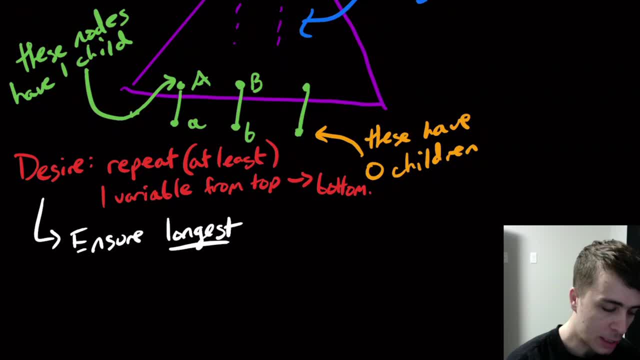 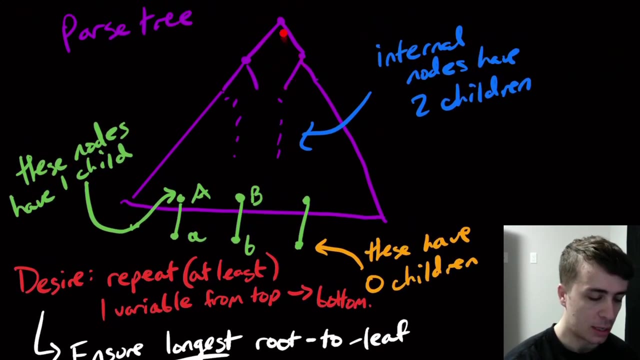 have some kind of repetition So ensure the longest route to leaf path. So that's how we actually write top to bottom. formally It's from the root, which is at the very top of the tree, and some choice of going from the top to the bottom, And the bottom here is the leaf. 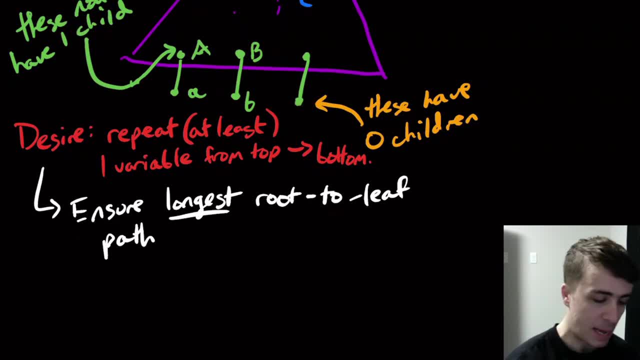 leaf because it's the bottom of the tree. So root to leaf path, ensure that the longest one repeats some variable. Okay, as long as we have that one working, then it's okay. So how are we going to do that? Well, if we actually try to look at this tree, 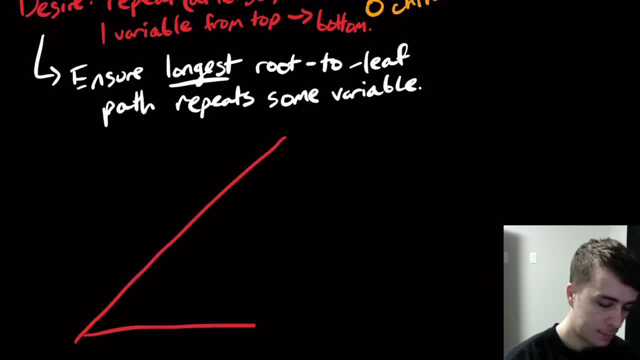 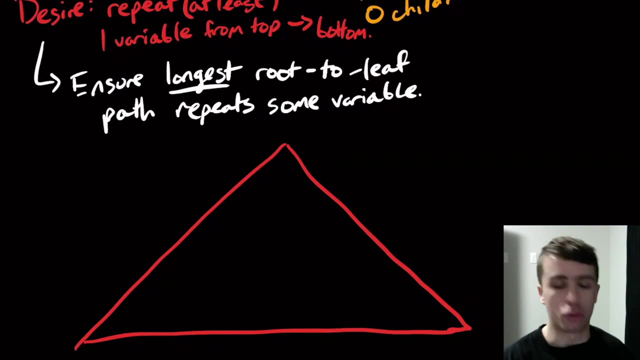 so here's our tree again, and it may not actually look like this. This is just what is called an artist's conception, So it may like be really short on one side and really long on the other one, because we don't know anything about the tree, But let's suppose that what we want. 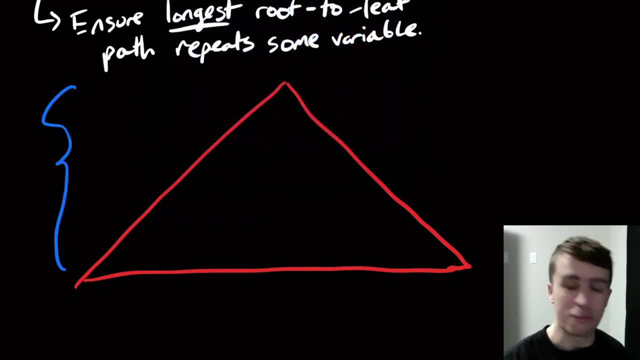 is that the the longest root to leaf path, which is what this is right here. So I'm ensuring that the longest root to leaf path is the longest root to leaf path. So I'm ensuring that the longest root to leaf path is the longest root to leaf path. 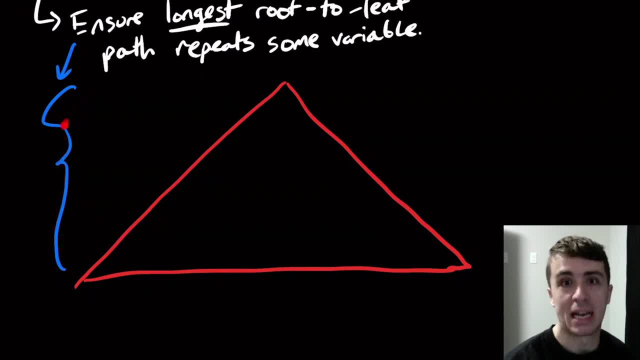 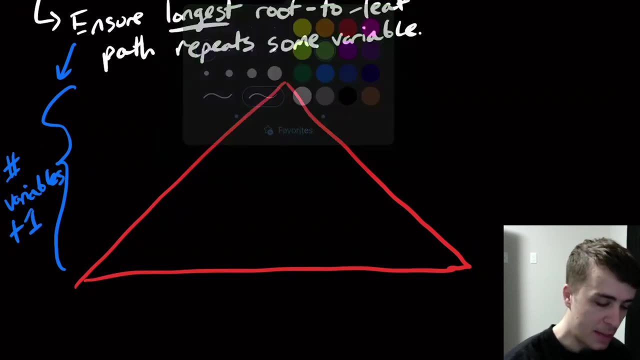 So I'm ensuring that the longest root to leaf path is whatever I'm determining this height to be. So if I make it so that this is the number of variables plus one, then whatever the longest root to leaf path is, let's just say it's this green one, right here. 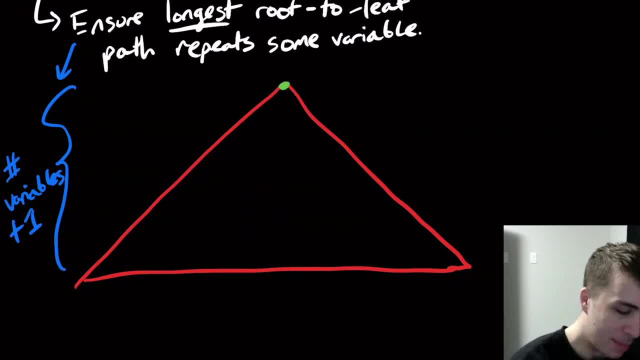 It's just: uh, oh, it doesn't, doesn't come up, It only goes downwards. So let's say it's this one and I'm going to actually notate that. So this, this path, is this one right here. In fact, there could be multiple, So it may be that there are multiple longest paths. 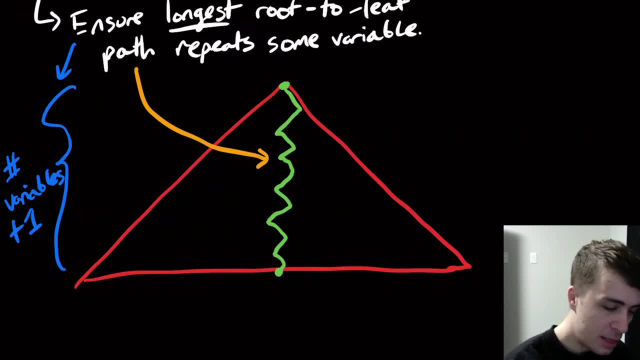 but I'm just picking one of them. So then this repeats some variable, because if? if it didn't, then let's suppose that there are no repetitions of variables from the top to the bottom- Then, because we have this being the number of variables plus one, 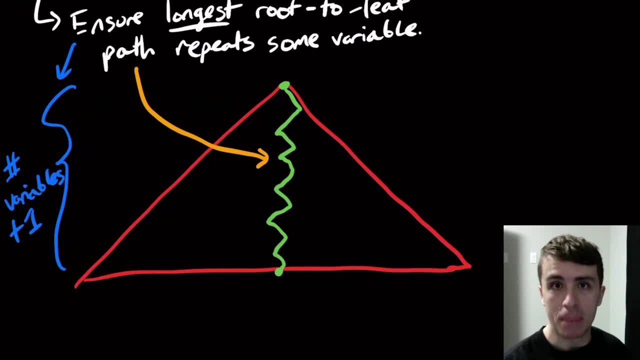 then that can't possibly be by the pigeonhole principle. So if we didn't have a repetition, then that means that we have some variable a, let's say right here, and there's no occurrence of variable a anywhere. but we have number of variables plus one pigeons and we have 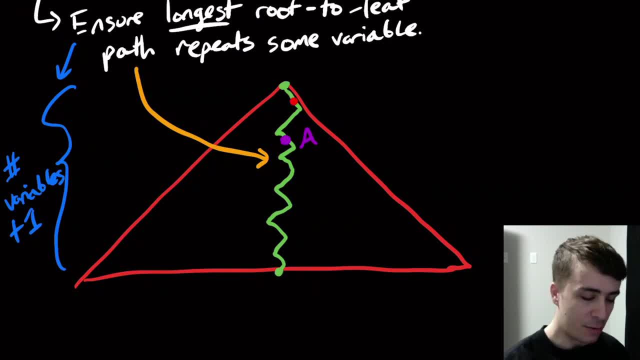 just the number of variables: number of pigeonholes. So we have a number of variables plus one pigeons, and we have just the number of variables: number of pigeonholes. So we have more variables that we see going from the top to the bottom than there are variables. 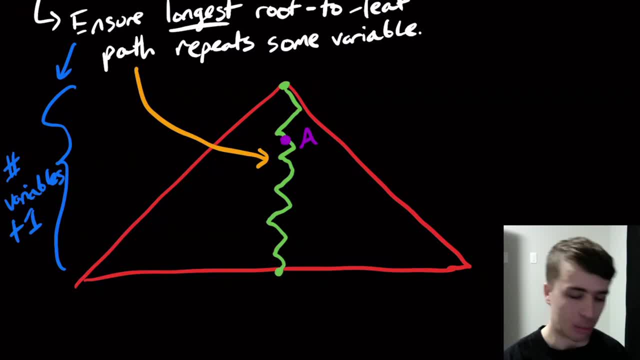 which means that there must be a repetition somewhere. So let's let then a be the variable that repeats. You can actually, you can actually ensure you can actually do slightly better than this, because the variable s can't repeat here, because s never appears on the right hand side. 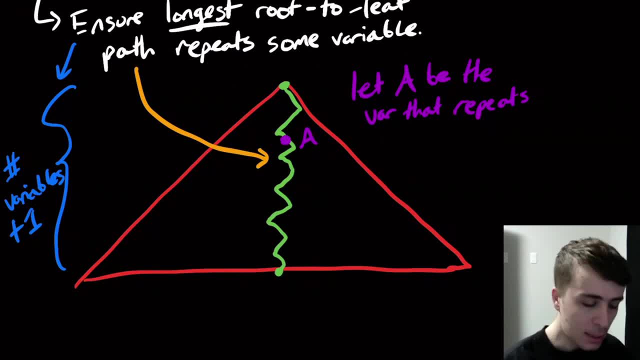 of a rule because it's in cnf, but this is sufficient in order. and let's say that a is the variable that repeats, So a appears here and then somewhere else a appears again. Well, what does that tell us about the string w that we have to generate down here? So this is the string w. 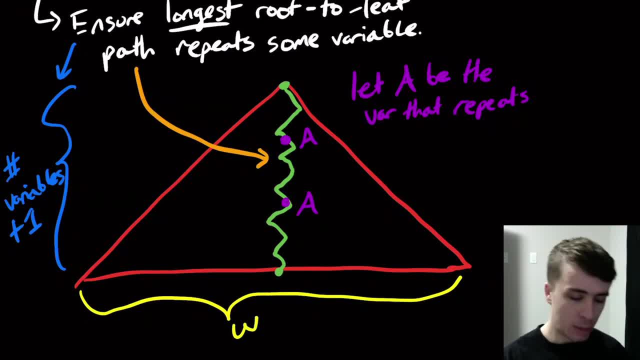 Well, we know that the tree is binary, so the length of w is going to. as long as w is at least two, to the power, the number of variables plus one which is the height of the tree, then that's sufficient, And this only will happen if the tree is what is called a complete. 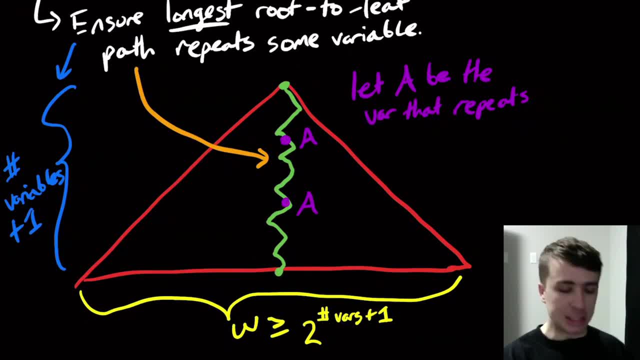 full binary tree, which means that it doesn't stop early at some point. here It goes completely down and it's exactly the same level all the way around. So as long as it's at least this amount, then that means that there is. there must be some way to get from the top to the bottom. 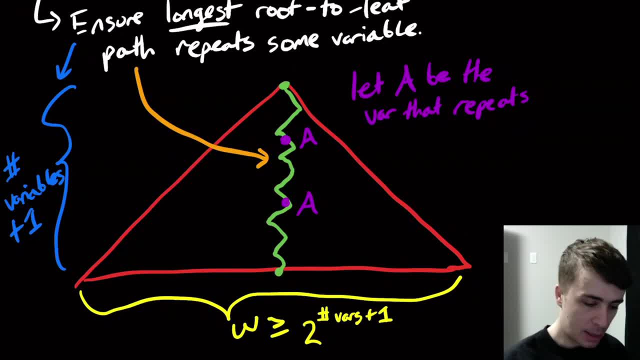 with a repetition somewhere. Actually, I think I need a plus 1 here to ensure this, but it doesn't really matter, because we won't actually use this. As long as this number exists, given the grammar, then we're okay, which is all that we need. Okay, so let's try to analyze this a little bit. So I'm going to go through the 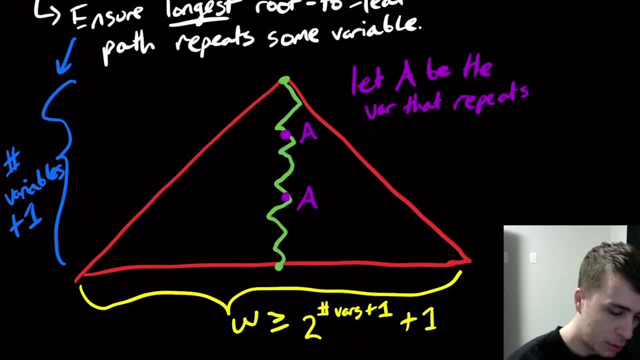 I'm going to- oops, I am going to- slightly modify this so that I have some room in the tree itself. So we know that the only variable in a grammar, that's in C and F can, the only one that can make epsilon, is the start variable. 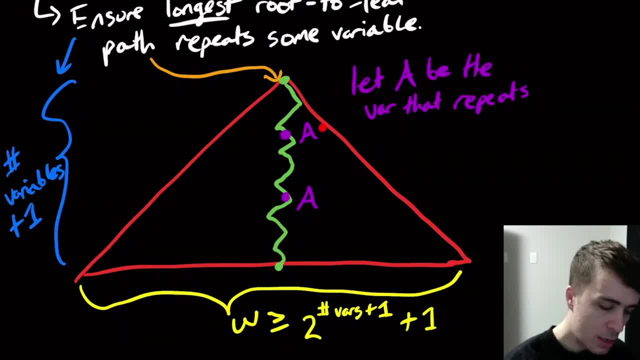 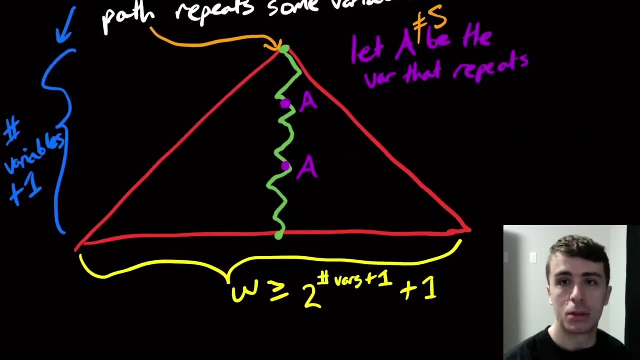 No other variable can actually make it. So we know that this variable A, because it repeats, can't be the start variable. So let me notate that. So this is not the start variable, which means that, oops, which means that A itself must generate something of the string. 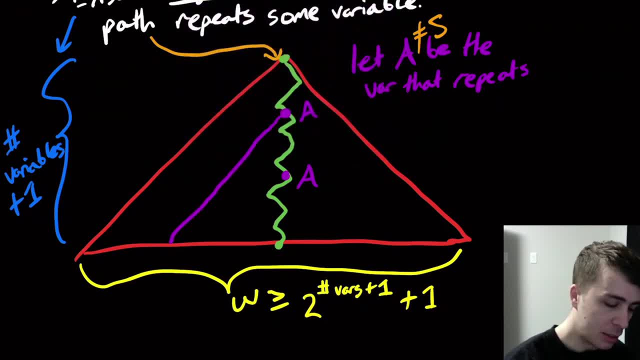 So let's look at what it can actually generate. So it generates something of the string, And the bottom A, of course, is also not the start variable, So it also makes something of the string too. By making something, I mean it makes at least one character. 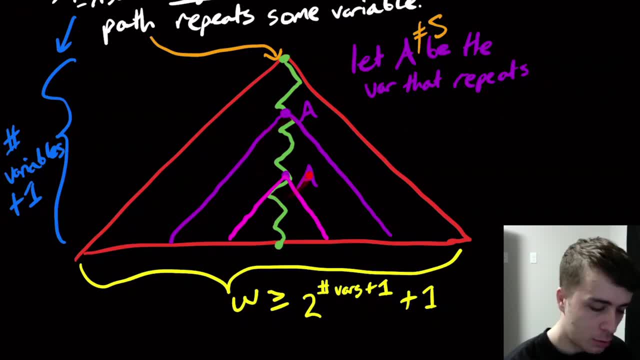 That's what I mean by that. Okay, so what do we actually do with this? What am I going to do? I'm going to move this down a little bit And I'm going to name each of these pieces. So this part right here, I'm going to call the U piece. 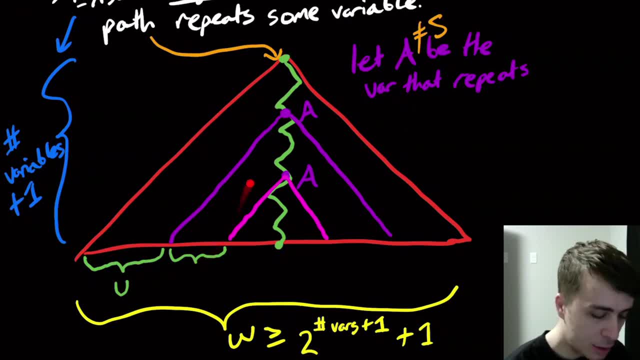 This one right here is one that the top A produces but the bottom A doesn't, And I'm going to call that V. And then this final piece, which is the part that only A will generate, I'm going to call X. 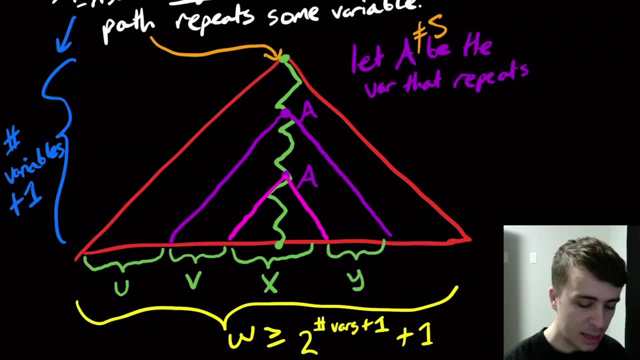 The other side is going to be Y and the other part, the very last part, is going to be Z. Okay, So the string that we generated is W, but I'm decomposing it into five pieces: U, V, X, Y and Z. 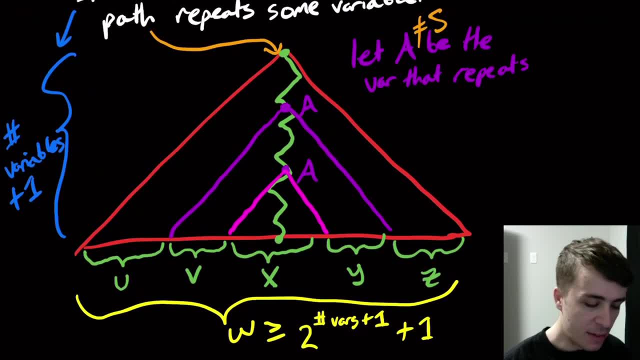 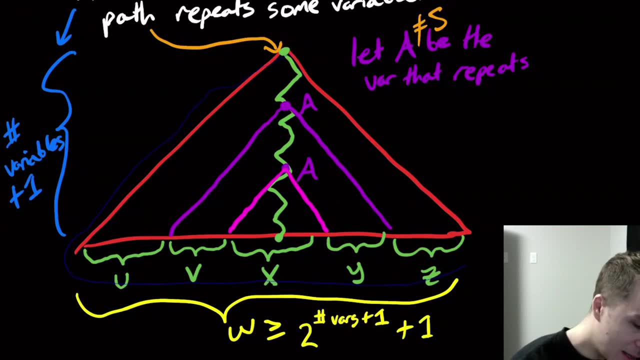 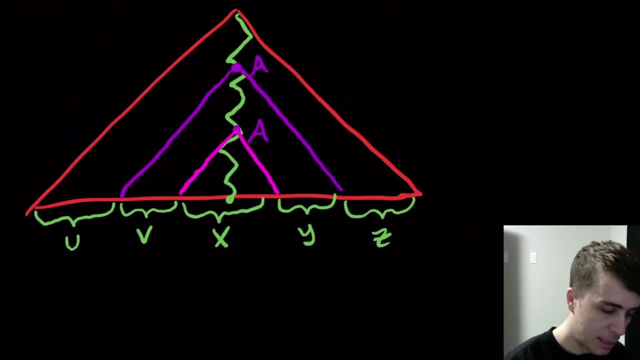 So how can we actually use this to our advantage? So what I'm going to do is I'm going to attempt- Quote, unquote attempt- to copy this tree down so we can analyze it a little better. So let's actually look at this tree a little bit. 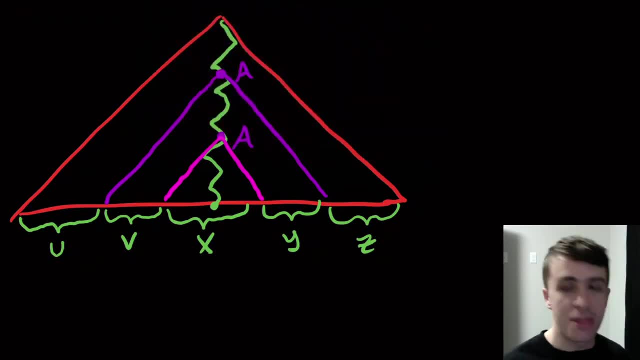 So let's try to understand what the variable A could actually make, Only A itself. So A clearly can make the X part, because it's just this variable A only making the X part, Through possibly many rules that are being applied here, But eventually it makes X. 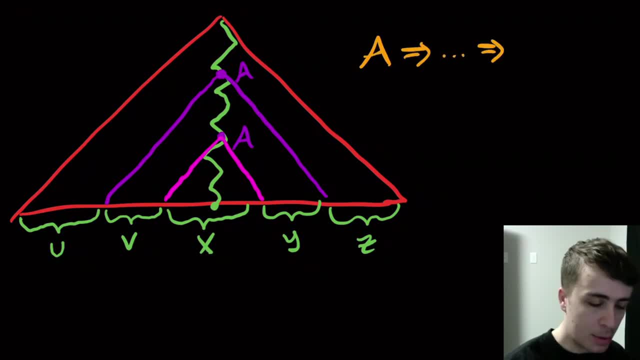 So A can eventually produce X. And I'm going to do a slight simplification to say here: when I say double arrow going right like this with a little star on top of it, that's the same thing as saying applying a bunch of rules to get the thing on the right. 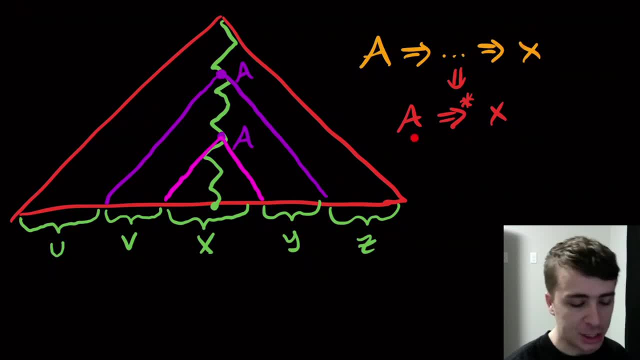 So applying a bunch of rules to get X. I'm just shorthanding it this way. Okay, So then. but if we look at one level up right here, we see that A also makes V X Y, So A will eventually make V X Y, of course. 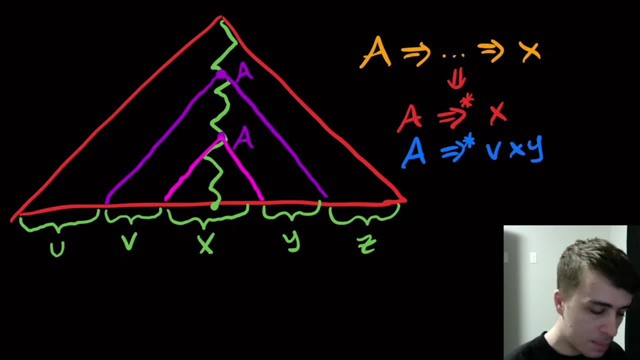 What else can we say? But, more importantly, we can use the recursive structure of context. It's free grammars to say This: A right here at the top can make the V part And then whatever the A part actually makes. So we can actually combine these to say that A will generate V, A, Y. 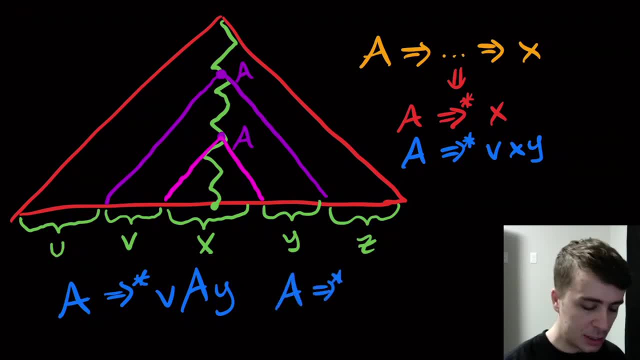 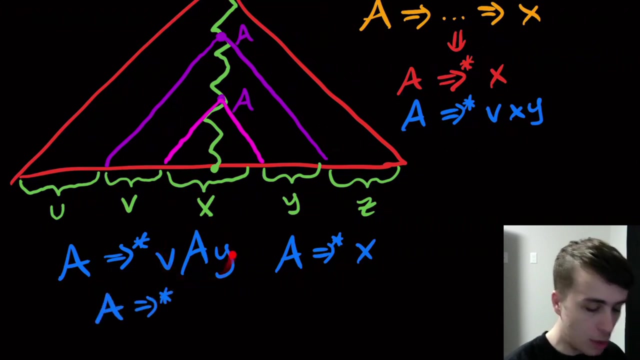 And also A generates only X. Okay, So this actually tells us something important about A. Okay, That we can actually repeat some structure of these V and Ys Namely, it will also generate, if we apply this one right here over and over and over, as many times as we want. 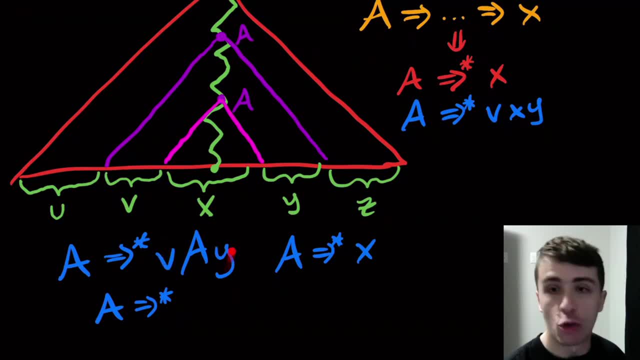 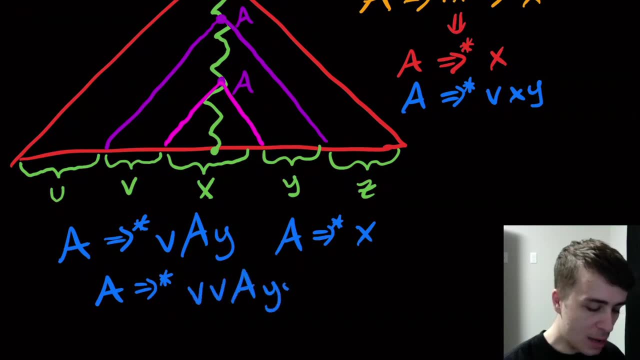 we will get a V on the left side and a Y on the right side, So what we'll eventually get is V, V, A Y, Y, And then eventually, So we can actually make three Vs A three Ys. 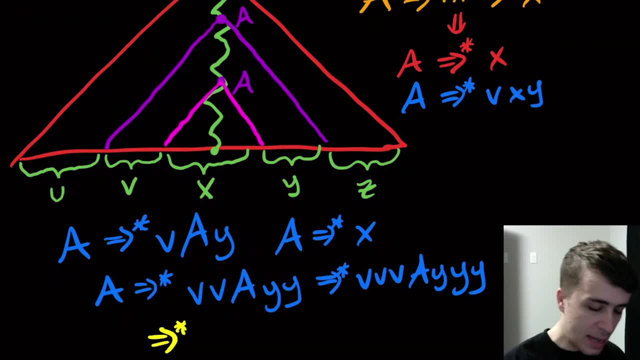 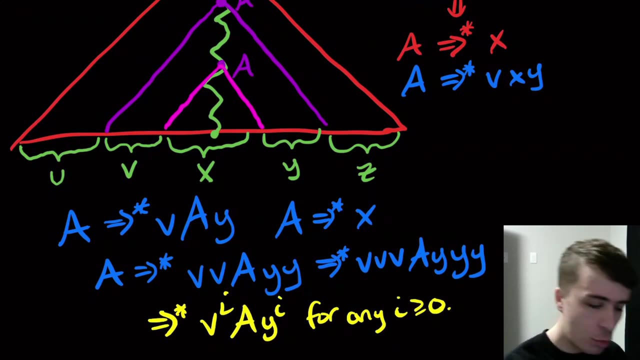 And you can see where we're going with this. We can actually get V to the I, A, Y to the I for any I, at least zero Okay. So it's kind of similar to the regular pumping lemma, But here we have two pieces where the exponent on both of them is identical. 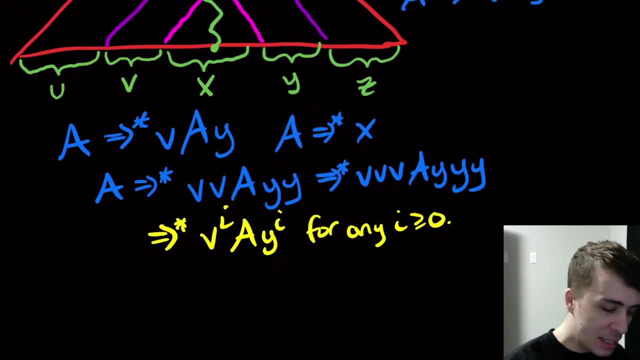 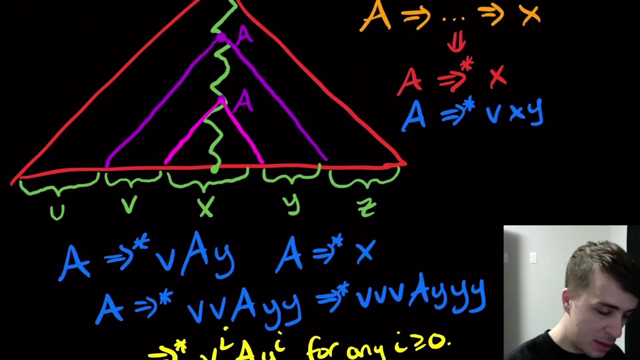 Okay, Okay. So then if that's the case, what we can do then is we can have the start variable, not A. the start variable can make- well, it can make the U piece And then anything that the A could generate, because this A right here is representing this A right here. 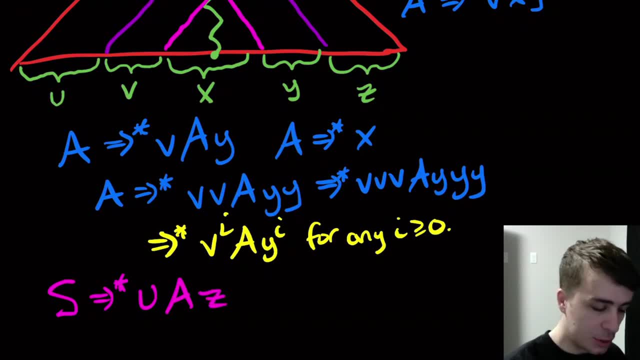 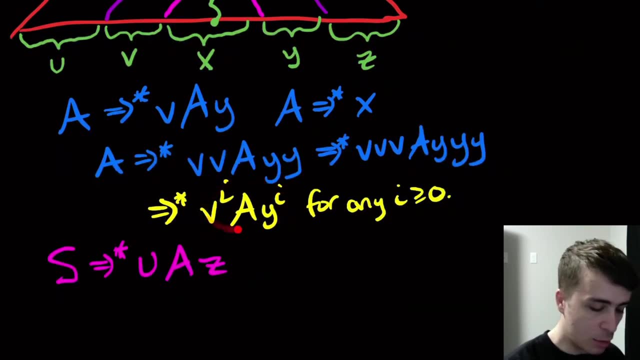 So, and then with the Z part at the end. So it's the U piece plus whatever A can make, And then a Z. But we already know what A can make, which is this. So this is: we can also generate U, V to the I, A, Y to the I, Z, just by substituting A here with this piece, right here. 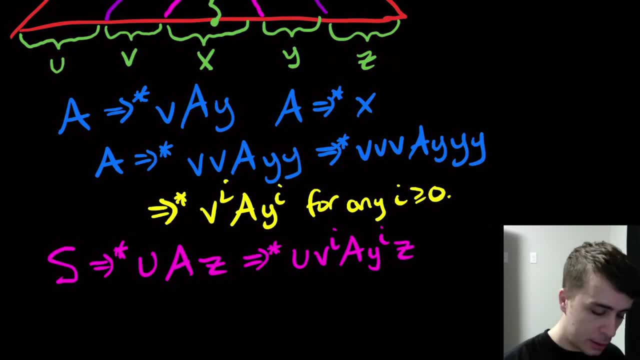 And also we know that A can generate X. So at the end of the day we can say that S could generate U, V to the I, X, Y to the I, Z, Z, for any I at least, zero Cool. 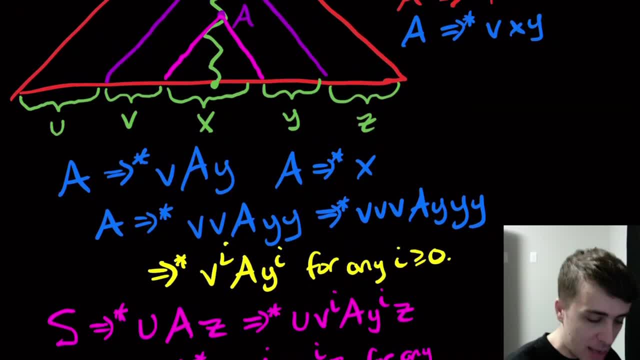 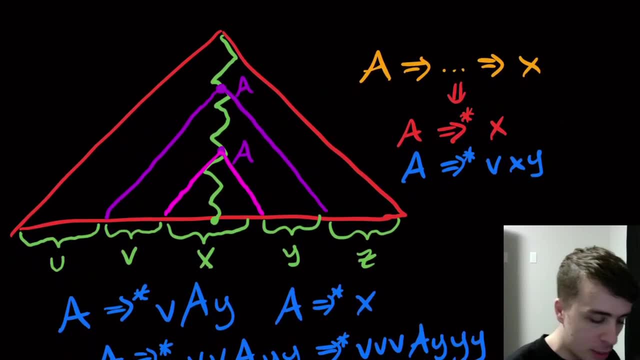 So pictorially. what does this actually mean? That means, yeah. so what does this actually mean in terms of the parse tree? What it means is that if I copy and paste this big A parse tree down to where this second one is, 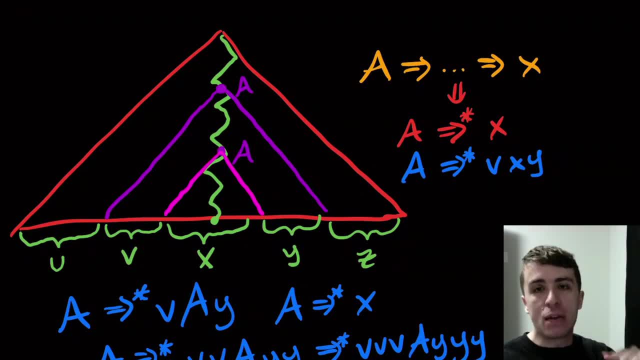 then we will get an additional copy of V and Y, And this X went away when we pasted it back in, But we'll get it back because we're copying and pasting this whole thing, which includes the X. So we'll never get an additional copy of X, but we'll get one copy of V and Y each. 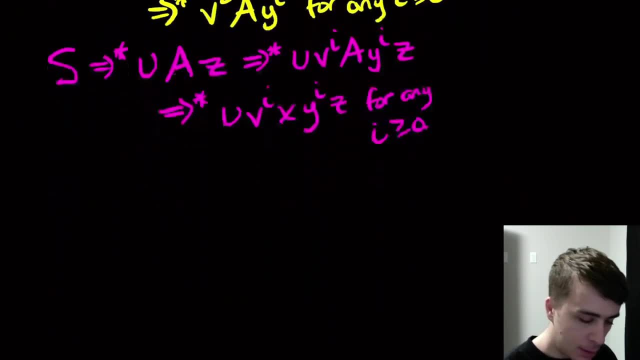 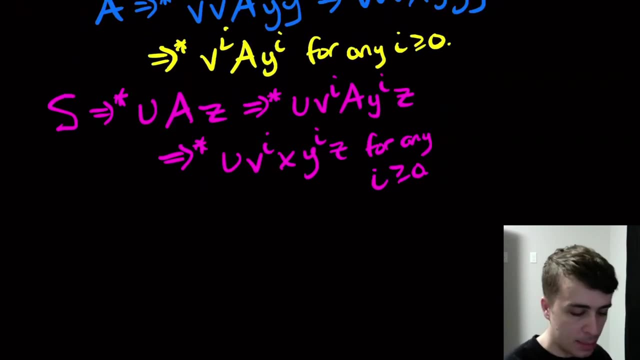 Okay, So that's kind of nice, But let's try to analyze this a little further. So we saw in the regular, We saw in the regular pumping lemma, that the part that had the exponent had to be non-empty because it involved at least one transition. 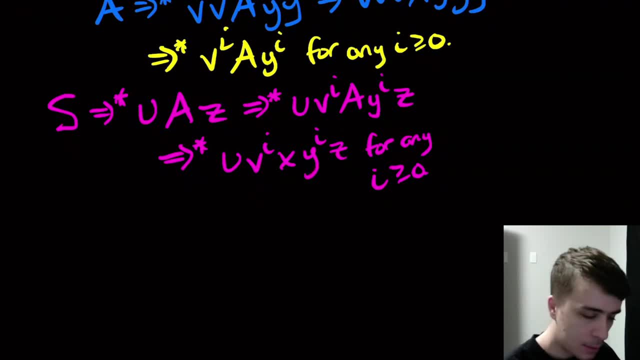 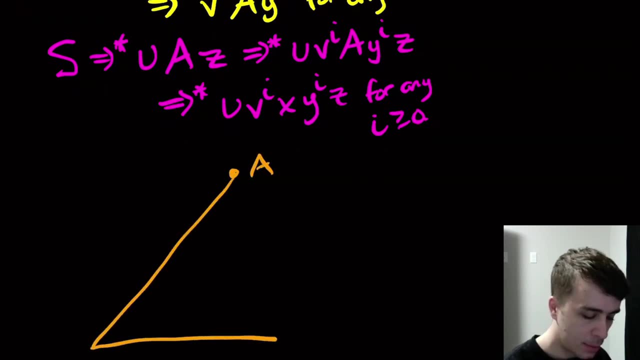 What do we actually do here? What do we know about V and Y? So let's try to analyze this. So I'm going to draw this a little bigger. So here's the top A here, And we have this path going to the bottom. 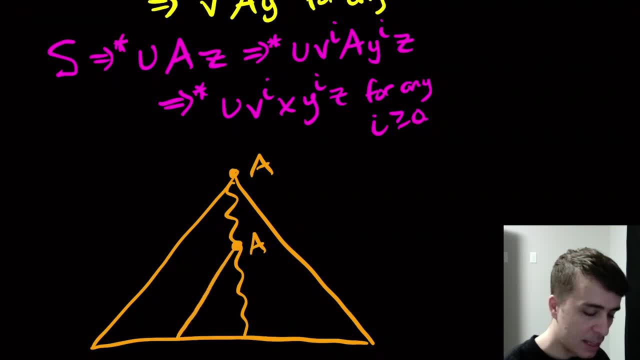 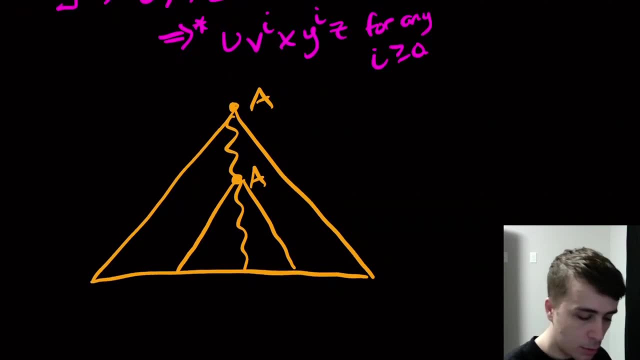 Here's the second occurrence of A, And it makes something of the tree like this. So what can actually happen? Well, the worst possible thing that can happen- quote unquote, to make V and Y as short as possible- is that this second A is as close as possible to the first one. 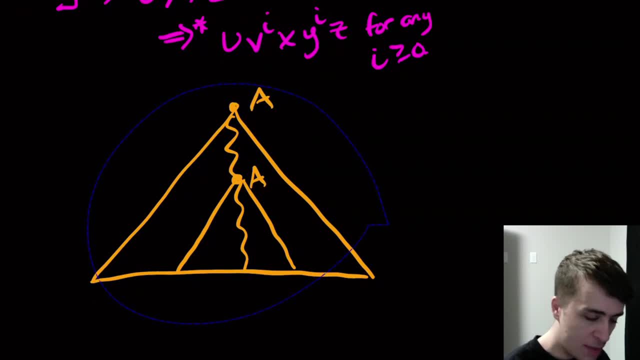 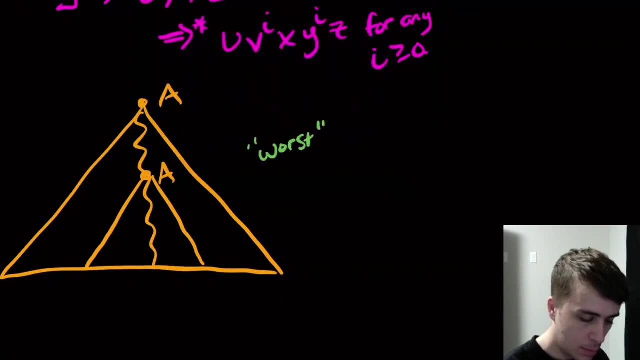 So let's try to analyze what that actually looks like. So the worst thing that can happen, Worst possibility, I'm going to call it, Which is that we have the variable A right here, the top one, And we have the second occurrence of A right underneath it. 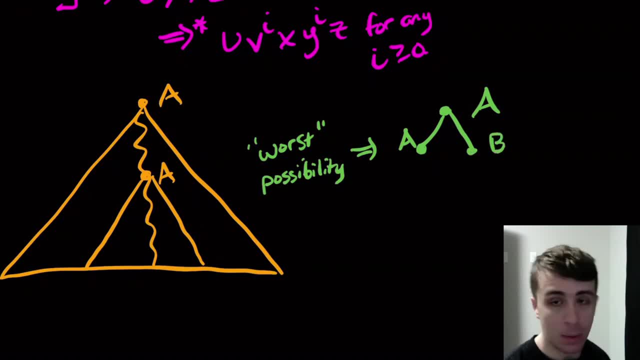 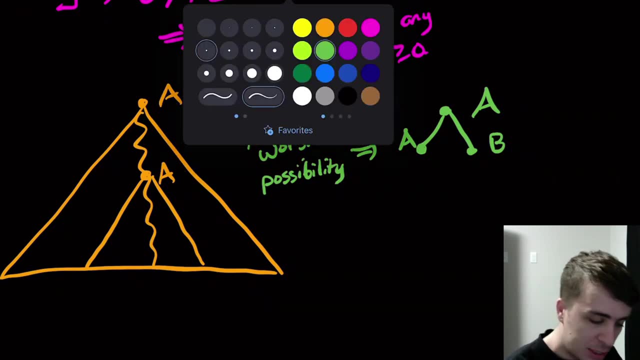 And then the right side could have some other variable, but I don't really care what. that is Okay, So that's the worst thing that can happen. So let's actually visualize what the tree looks like underneath this. So if I just draw the rest of the tree out, 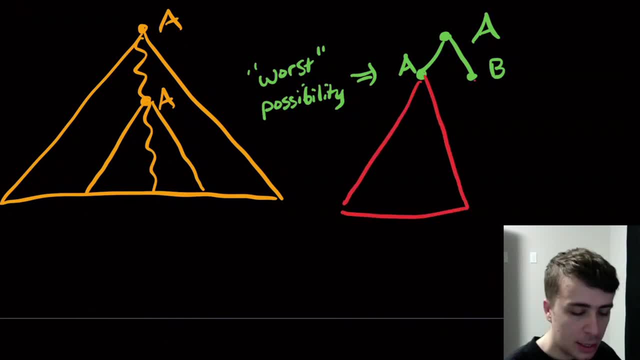 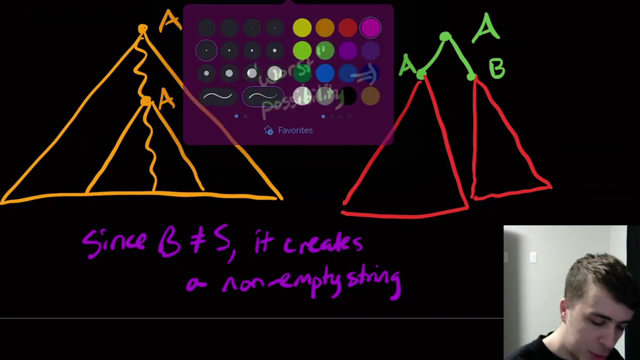 Okay, Note that the subparse trees under A and B do not coincide, So they're completely disjoint from each other. And also note that since B is not the start variable, it creates a non-empty string. So So So this part right here. yeah, I'm making sure it's on screen. 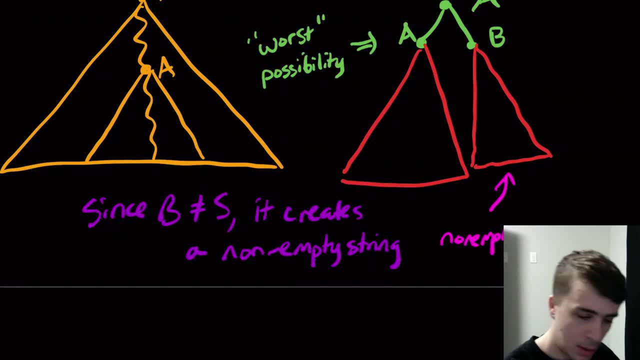 So this part is non-empty. The text went off there. Yeah, that part is non-empty. And well, this part right here obviously is non-empty also. but here's the key. See this part right here. if we visualize this parse tree over in this context, this non-empty piece is this one right here. okay. 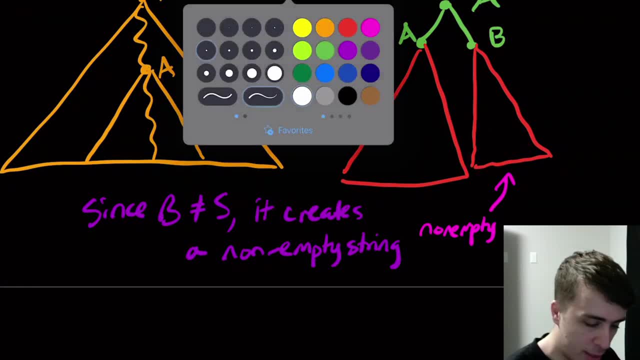 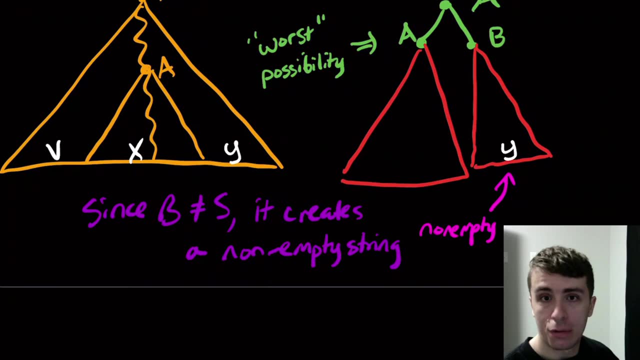 So this part is- let's actually draw it out- So this part's v, this part's x, this part's y, This part is y itself And this part on the left is: well, the v part is x. 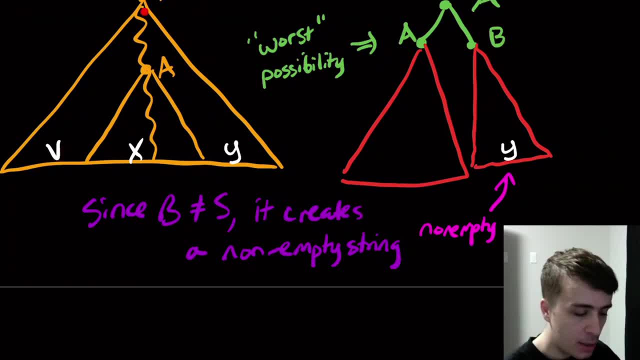 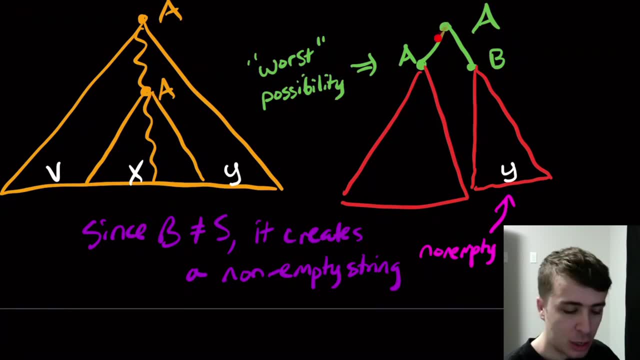 And this part is actually squished, because the v part is what is generated on the left side by the top a but not the bottom a. So it's, on the left, generated by the top a but not the bottom a, But because they coincide, it is the case that v on this side must be empty, believe it or not. 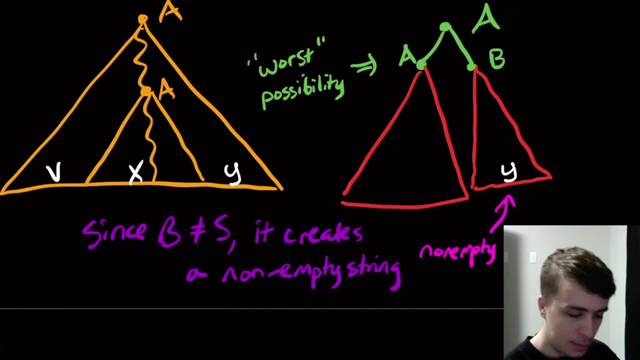 So in this case v is empty. So what really is over here is just x and nothing else. So in this case the v part actually is empty. And if we flip the roles of b and a here, well, the roles of y and v reverse, it'll actually be that y is empty and v is non-empty. 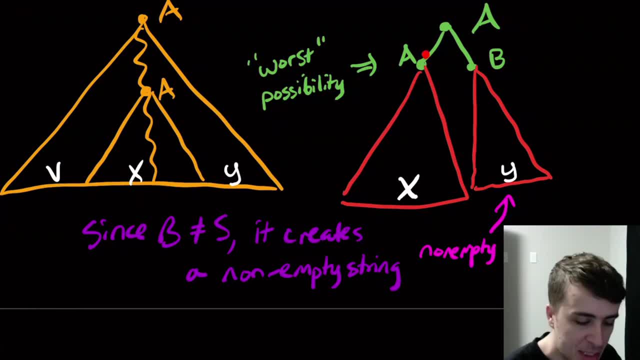 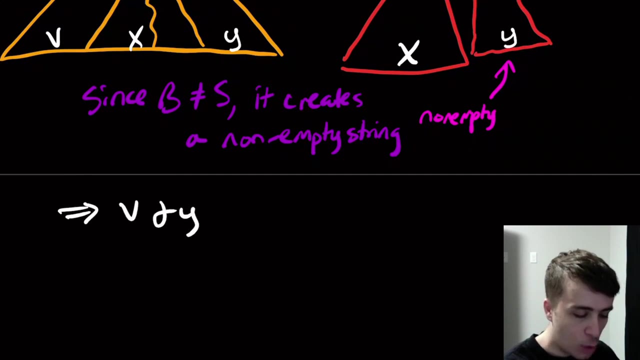 But the key is that, because this is only on one side of the two, it can't be the case that v and y simultaneously are empty. So what we'll get out of this is that v and y cannot be simultaneously, and yes, I've learned how to spell simultaneously, right. 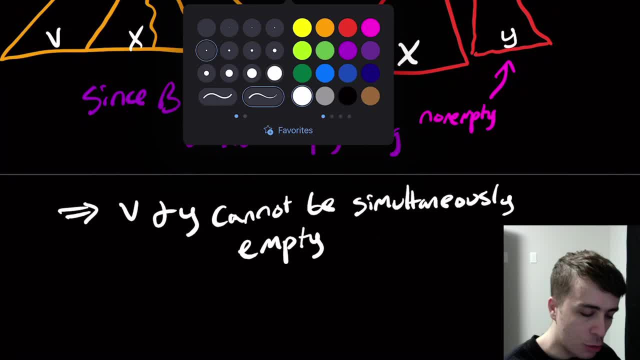 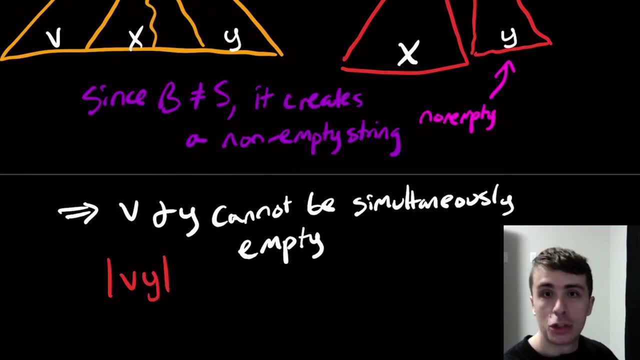 Empty. So one way that we actually write this- and there are other ways you can do it too- the length of v, y together. So this is not in the original string because the x part's separate. It separates them, but it's just considering those two pieces together as a different string. 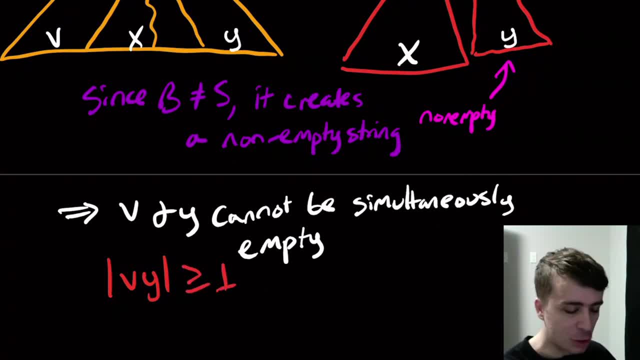 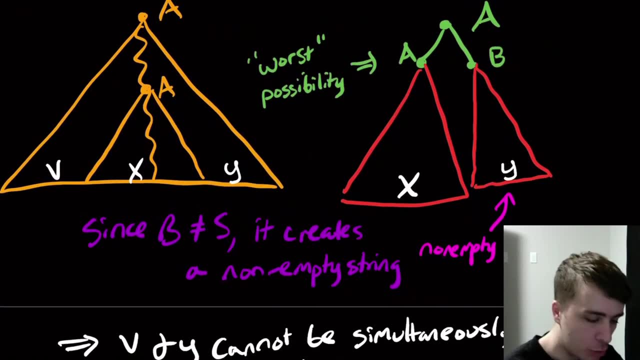 So v and y together, its length is at least one. One of the two at least is non-empty. It could be that both are non-empty because this picture right here looks like the v and the y part are non-empty. But when it's as close as possible to the other occurrence of a, then one side is going to be empty. 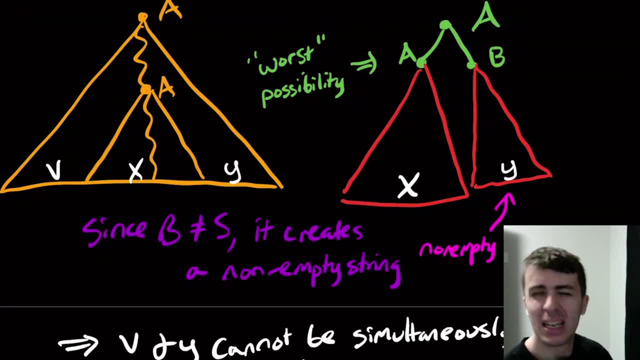 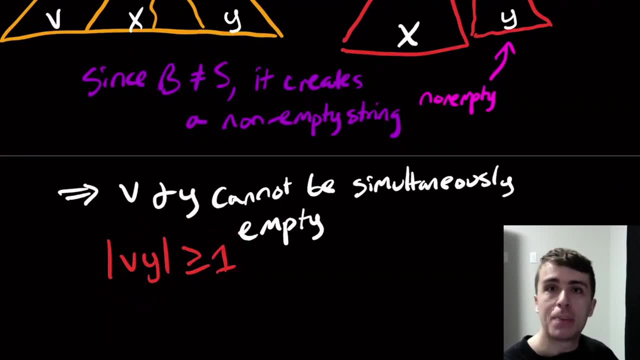 and the other one has to be non-empty because the grammar is in c and f. Isn't c and f? awesome, Anyway. so that tells us the other condition and, as you might expect, the pumping one that we did before the five pieces, one and this one are all that are actually needed, but in order to make the proof, 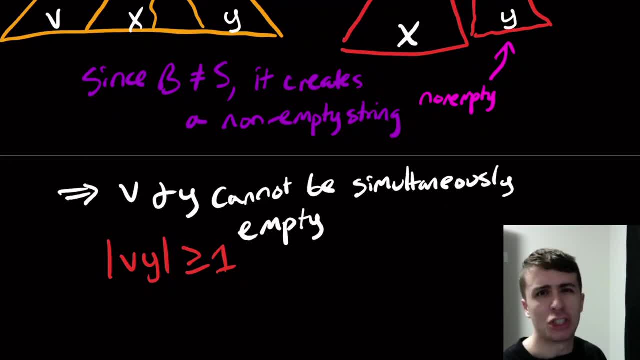 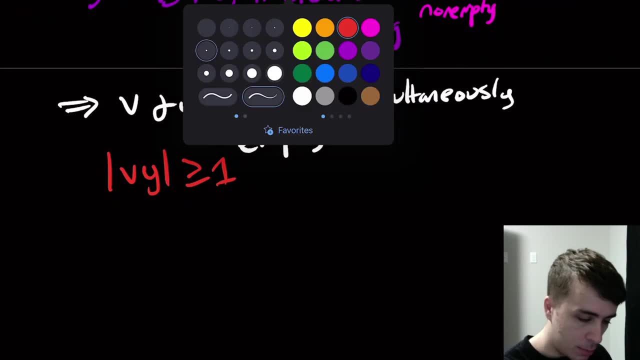 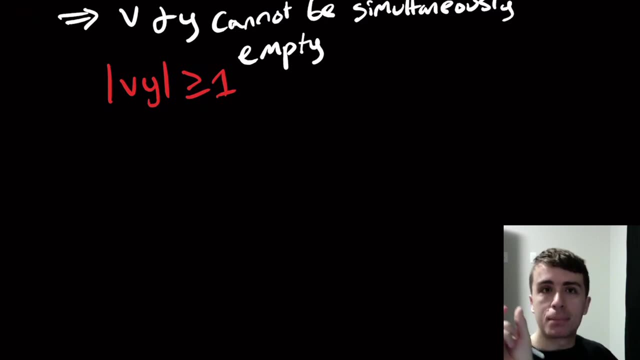 significantly easier for showing some languages not being context-free. we need a third condition. So what is this third condition? So what we can do is remember, when we were talking about the regular pumping lemma, we required that the pumped piece, which is the the y part, to be as close to the beginning as 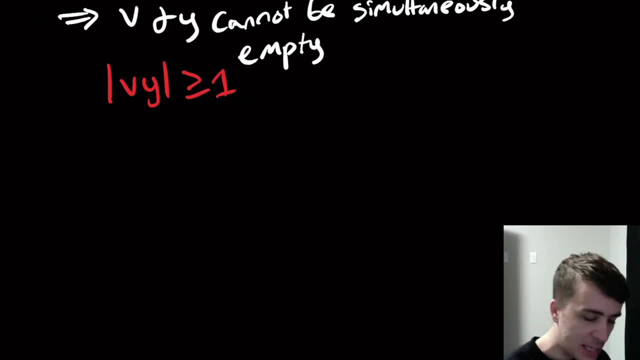 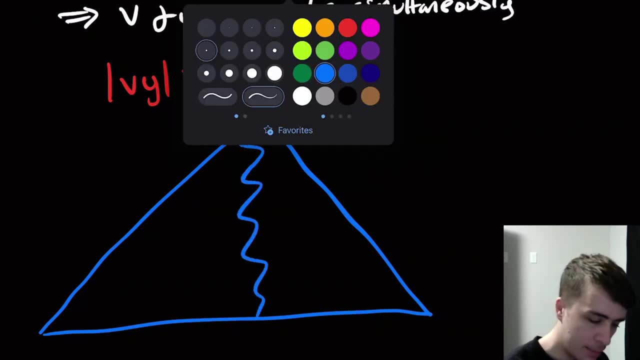 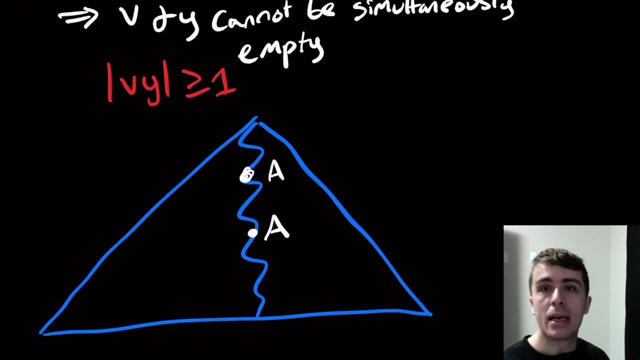 possible within the first p characters. The idea here is that if we have these variables repeating from the top to the bottom- so let's say that a is here and then a is here- then what we're going to do here is we're going to assume that we are talking about the. 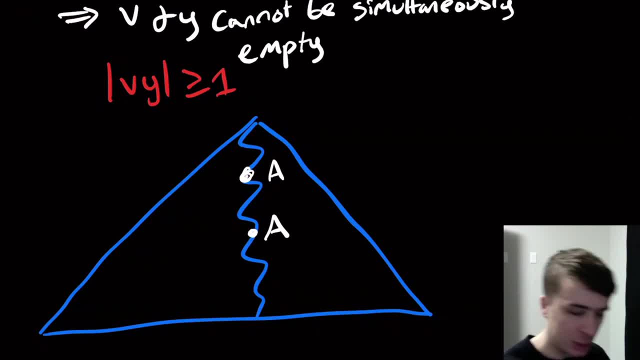 repetitions as close to the bottom as possible. So let's try to write that down. So let's say that these two are the repetitions. although it doesn't look like it, these are the repetitions closest to the bottom, or the leaves of the tree, same thing. So why is that? Why do we want to do that? 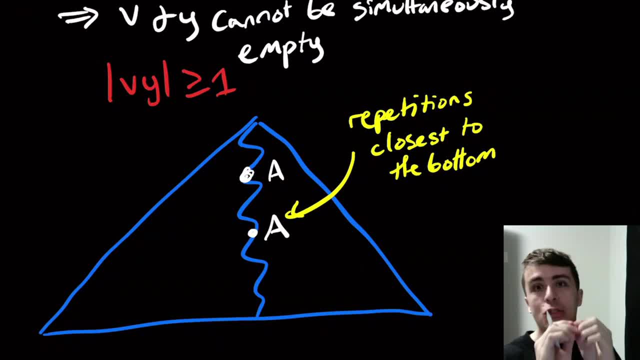 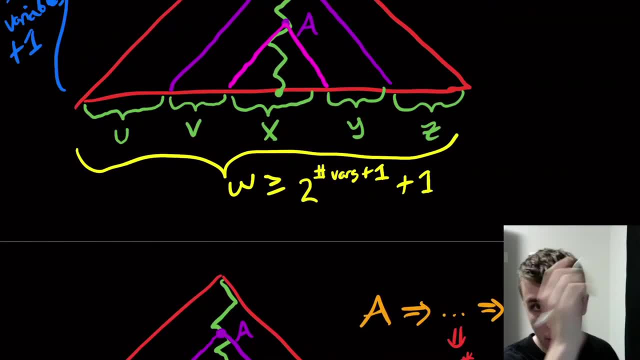 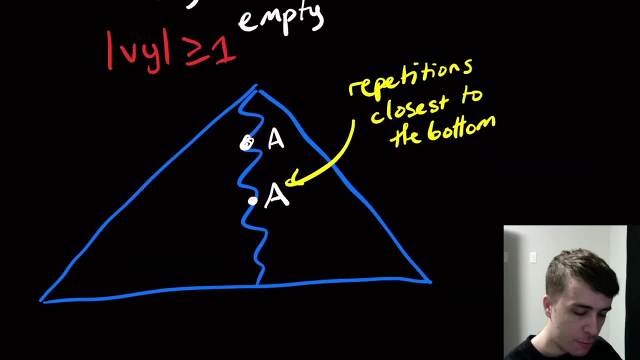 Suppose that the string that we're making is really really big, like way, way, way more than this two to the number of bars thing, Suppose it's way bigger than that, Then what we can do is if we focus on a piece of it like this right here, this repetition, if we just consider it, 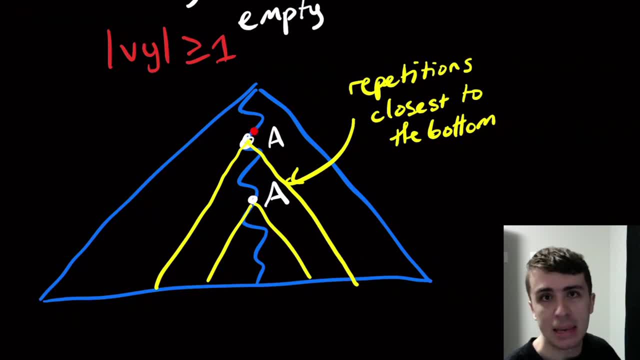 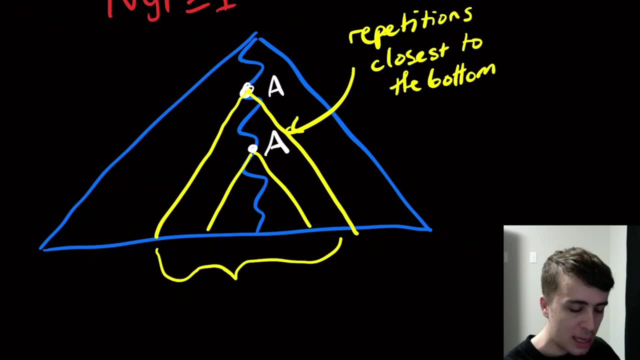 maybe at this variable or maybe somewhere else. we can just consider it at this variable or maybe slightly above it. what we can ensure is that this part, as long as it's at least two, to the number of bars plus one plus one, whatever. it doesn't matter what that number is, as long as we consider. 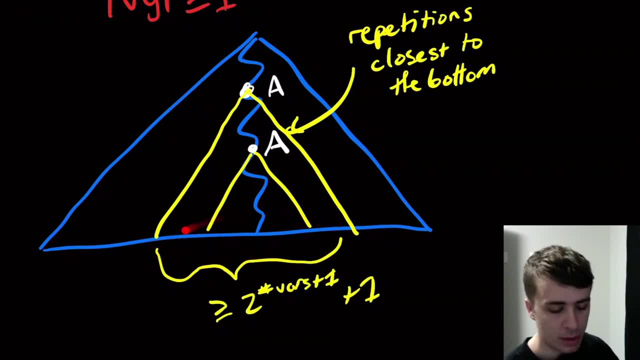 a subtree of, or at least a substring of, the thing that we're making. as long as it's at least this magic number, then what we can guarantee is that within the number of bars we're going to be able to make a repetition. So in the subparse tree right here there must be a repetition. So must 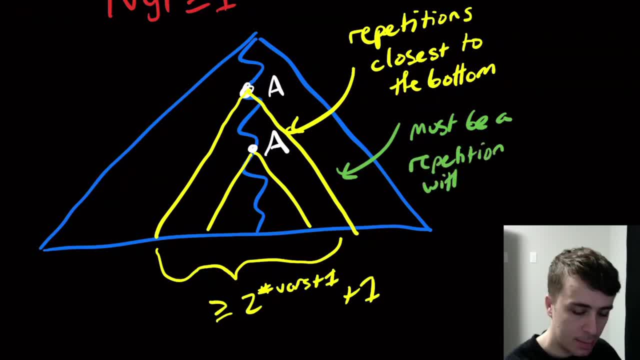 be a repetition within this subparse tree. Make sure it's all the screen. Okay, why do we want to do that? Well, remember that we want to establish some kind of repetition. So we're going to want to establish some kind of repetition. So we're going to want to establish some kind of repetition. 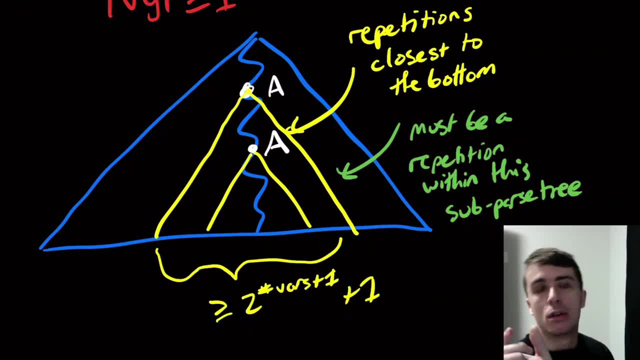 So we're going to want to establish some kind of this pumped piece is at most this magic number. So what we can guarantee is: well, this part is the v, this part's the x, this part's the y. Well, if we consider this part right here, then what we can guarantee is that, even at the worst, 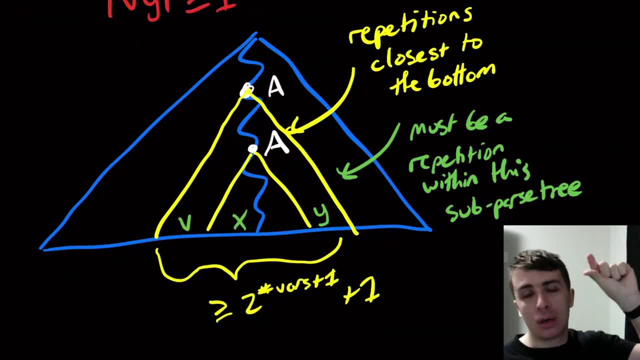 possible case. these two repetitions are as far, even though they're the closest to the bottom. they're really close to the bottom. So we're going to want to establish some kind of repetition, So we're going to want to register that as a repeating fraction of the whole. queroca saber. 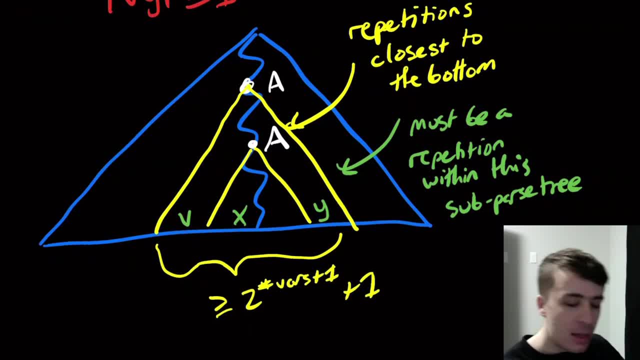 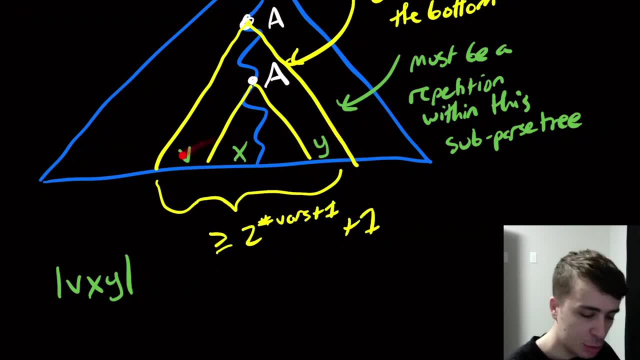 essentially So that's the very same thing at 15.. So we're going to have that as a acetate. They're really freedom far apart from the bottom. Then what we can guarantee is that v, x, y. 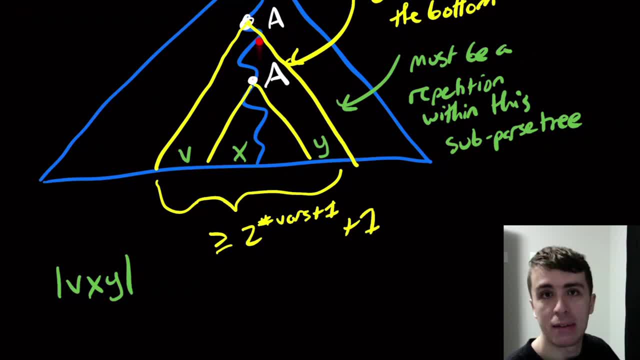 the whole thing, because this is what is generated by both of the pumps, I'm sorry, both of the repeating variables. this part is at most this magic number, Because it's the same idea as what we did for regular languages. This is telling us that this part right here, even if the string is huge, the part that 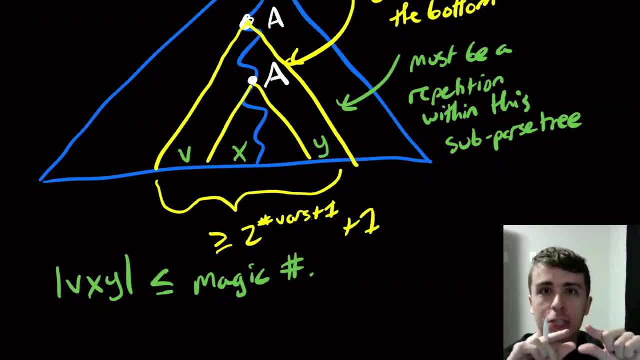 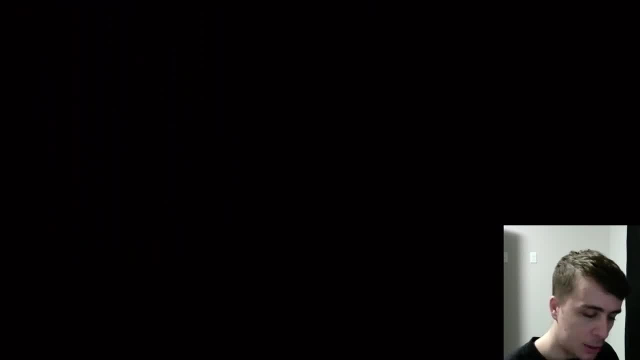 we will only need to consider is a very, very, very small piece of it, potentially compared to how big the string could eventually be. Okay, so what we're able to write down- because we just proved it- is the pumping lemma for. 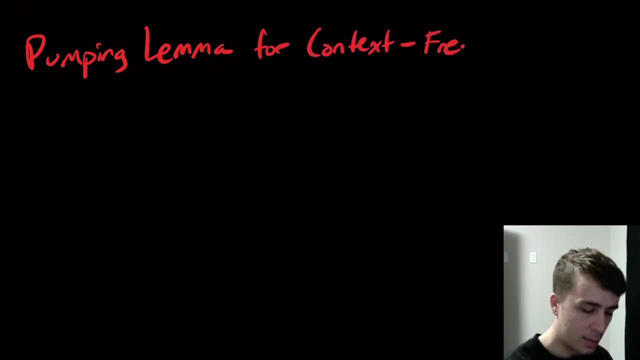 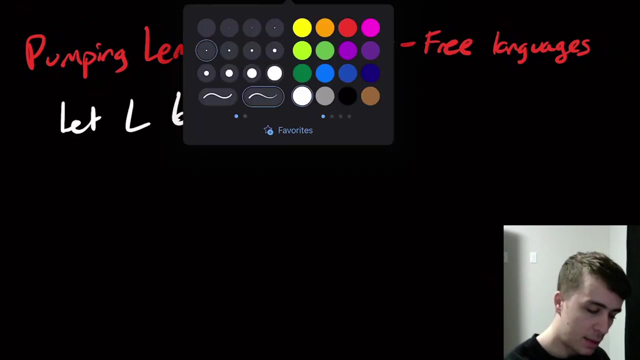 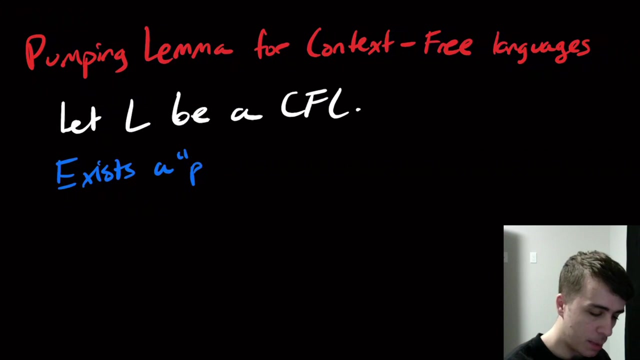 context-free languages. So the way that it starts out is almost identical. So let's let L be a context-free language. Then there exists a pumping constant- if I can spell pumping, that'd be good. pumping constant P for L. Then all that we need to do is so this P here is representing two to the number. 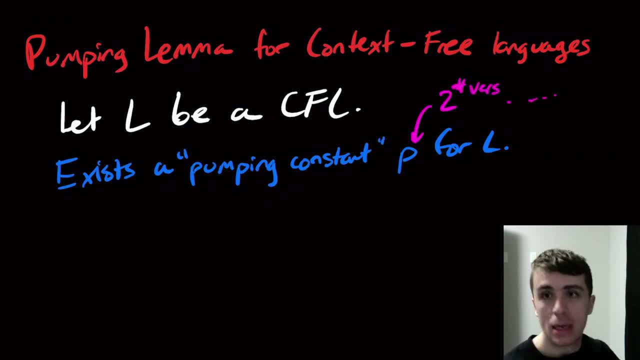 of bars in the grammar and whatever, although it doesn't really matter exactly what this number is. As long as it exists, given the grammar, then that's okay. Note that I'm not saying anything about the grammar itself, Because it's a context-free language. I know that there is a grammar for it. 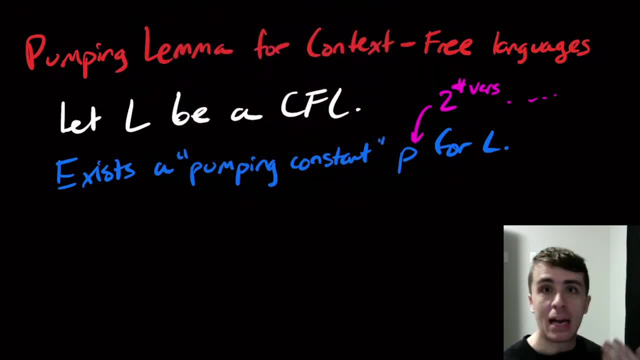 That's all that matters. So, then, what we need to do, as before, is we need to choose a string that is in the language, and long enough. We need it to be in the language, because we can't make a parse tree unless we have it. 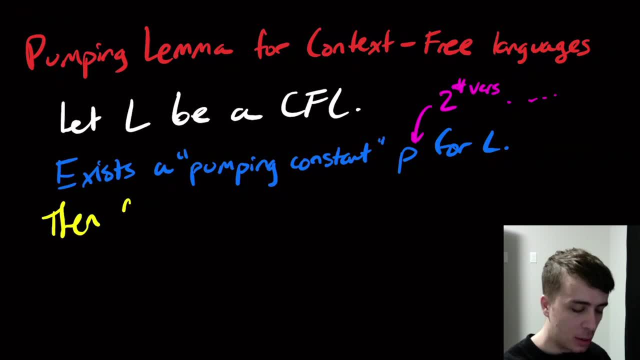 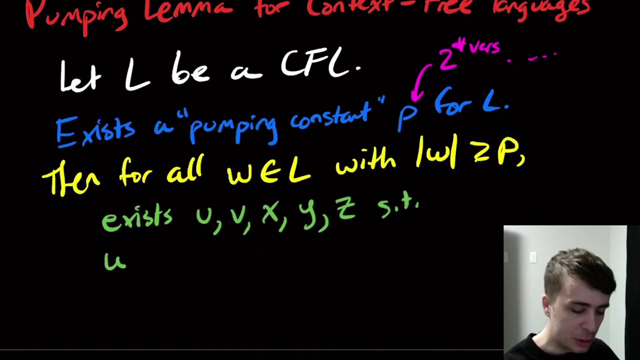 So, then, we need to consider, for all W in L, with the length of W, at least that magic number which is guaranteeing the repetition from the top to the bottom. Then there exists U, V, X, Y and Z, such that the string that we have, W, is equal to putting. 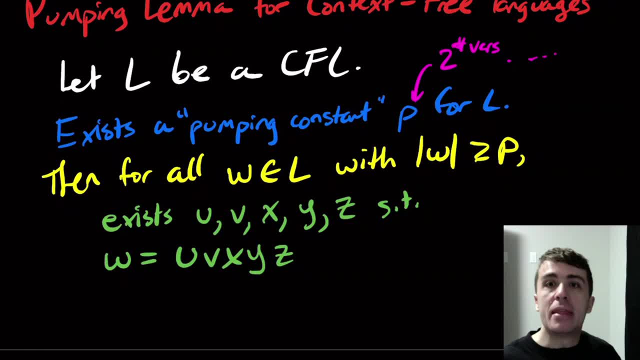 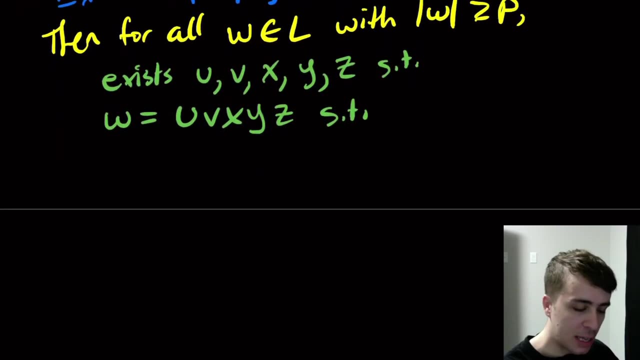 all those together. Why is that? Because we read the tree leaves from left to right and we will, yeah so remember it was broken into those five pieces. Okay, According to those three rules, such that. and then now, just like before, we have those. 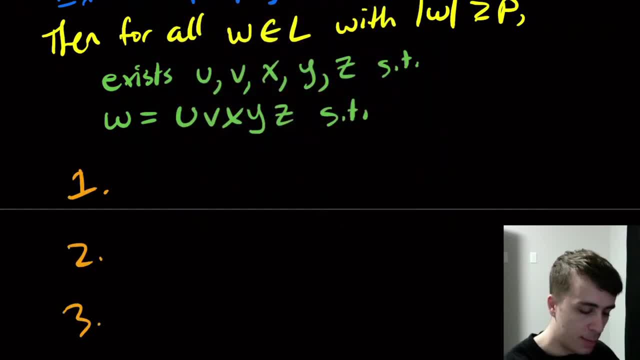 three conditions. So one, two, three. We will have that U, V to the I, X, Y to the I. Z is in L for all I, at least zero. We will have that V? Y together. It has at least one character.